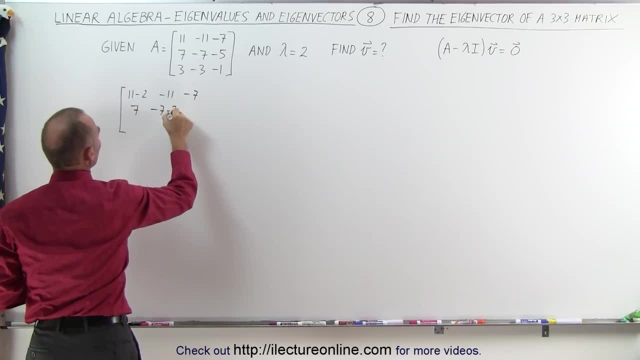 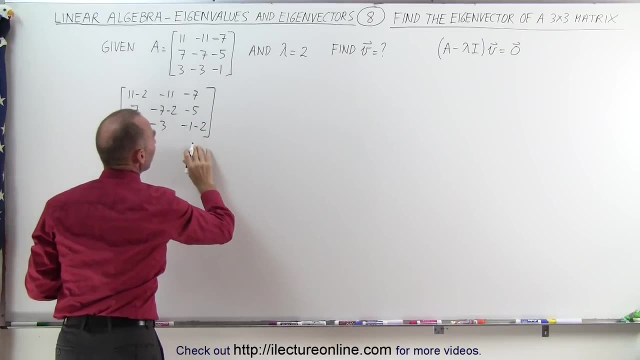 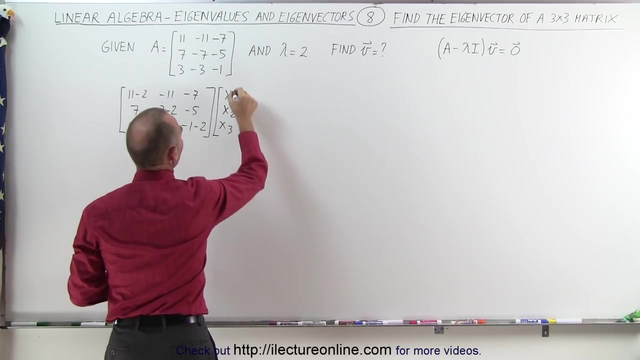 we have 7, minus 7, minus 2, and a minus 5, and 3, minus 3, and a minus 1, minus 2.. And then we take the whole thing and multiply it times the eigenvector x1,, x2,, x3, and that should then 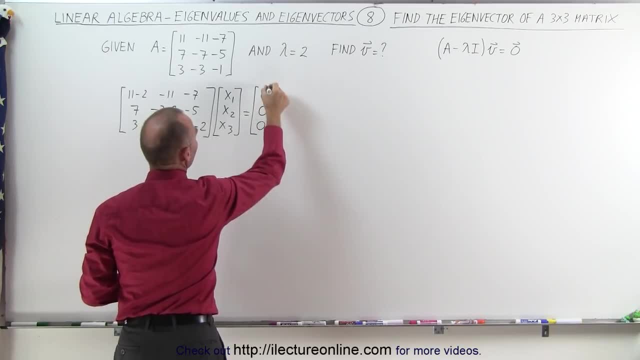 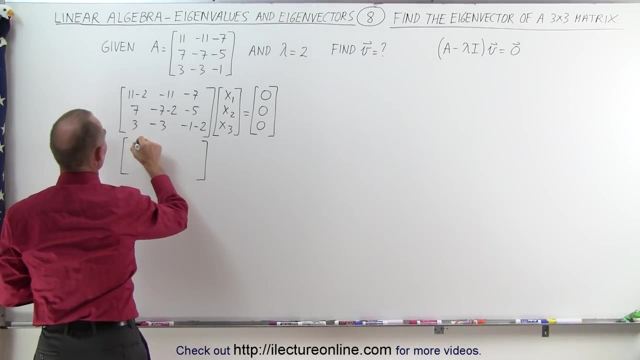 give us the null vector: 0, 0, 0.. All right, simplifying this so we can take a look at and see what we're dealing with Here. we have a 9, a minus 11,, a minus 7,. we have a 7, a minus 9, and a minus 5,, a 3,, a minus 3, and a minus 3,. 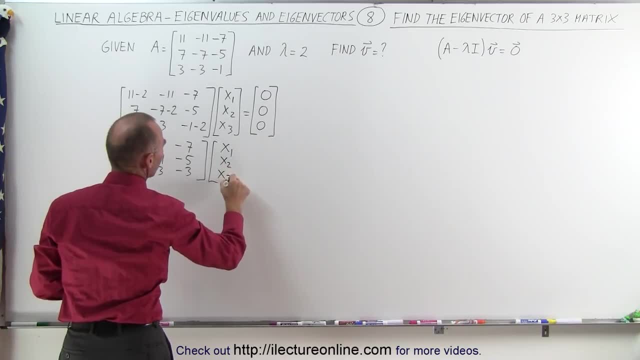 multiplied times x1, x2, x3, the three generalized variables, and that equals 0, 0, 0.. Now we have like a system of linear equations. Notice: here we have 9 times x1, minus 11, x2,. 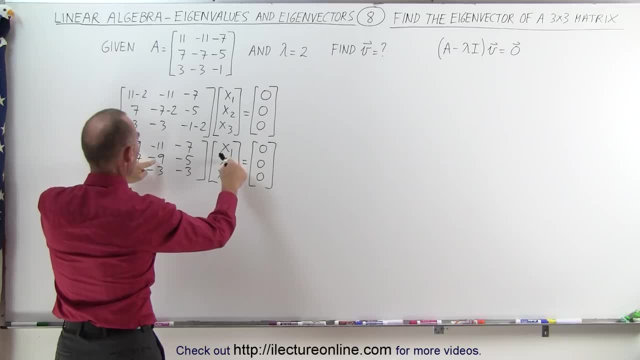 minus 7, x3, equals 0, 0, 0.. And then we take the whole thing and multiply it times the eigenvector 0, 0, 0.. We have 7x1, minus 9x2, minus 5x3, equals 0, and 3x1, minus 3x2, minus 3x3, equals 0. 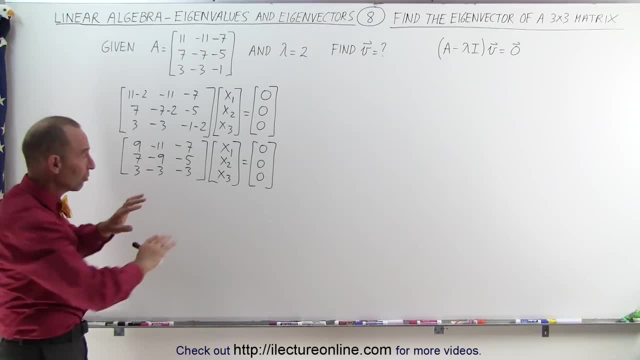 And we're supposed to solve for x1,, x2, and x3. That's how we'll solve this system of linear equations, And that will then be the eigenvector. The way to do that is to try and make these into zeros. In other words, we're going to write an augmented matrix. Let me do that now. 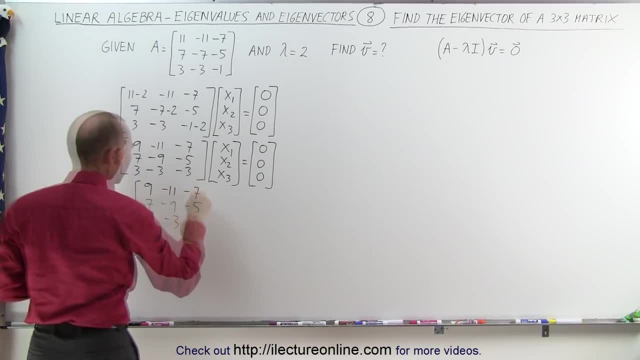 So we'll write a null, A minus 11,, a minus 3, and a minus 3.. The augmented zeros here, And if we turn these three elements into zeros, we'll be able to read the values for x1,, x2, and x3.. That's the reduced. 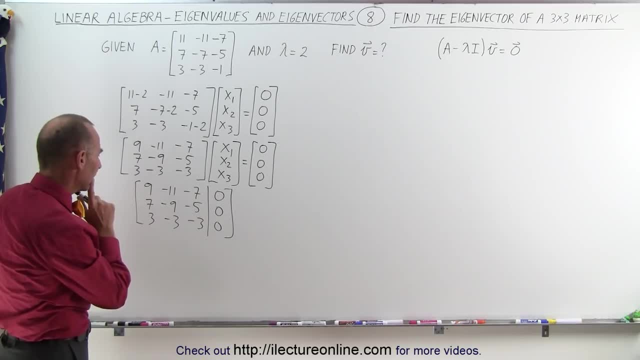 echelon form. So let's see here, The best way to do that is to move this to the top and this to the bottom and then divide that new row by 3 to get a 1 in this corner. So let's do that. 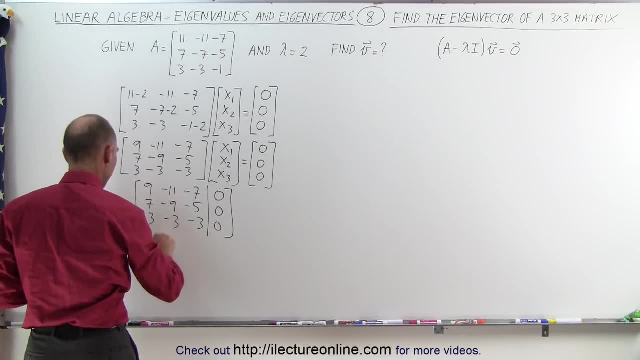 We're going to first interchange r1 and r3. And then we're going to take the new r1 and replace it by one-third r1. And if we do that, we get the following matrix: Let's see, Can I squeeze it in there? Let me go up here We have 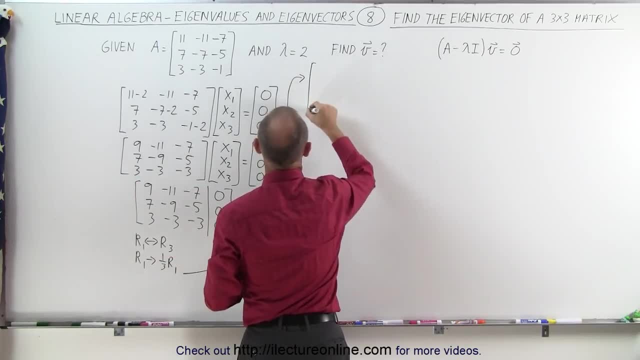 more room. So when I do that in the top, I end up with this row, but divided by 3. So this becomes a 1, a minus 1, a minus 1, and that's still 0.. The second row doesn't change: 7, minus 5, and 0.. 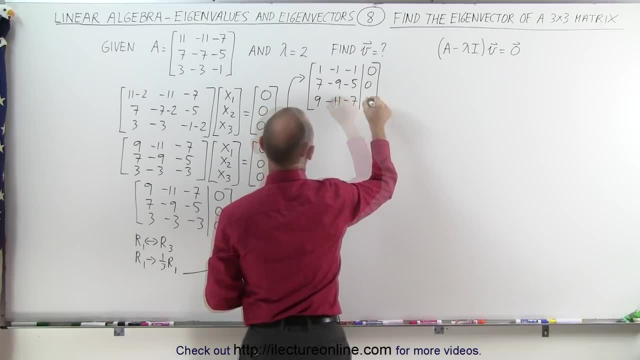 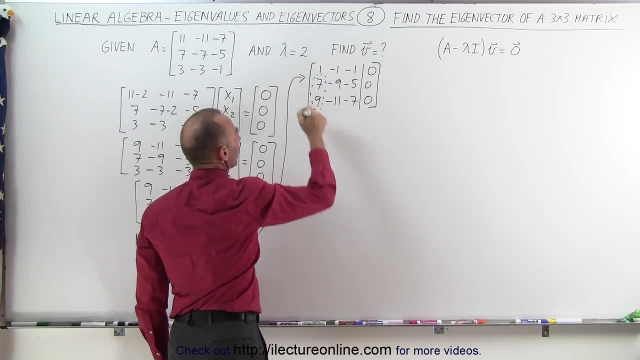 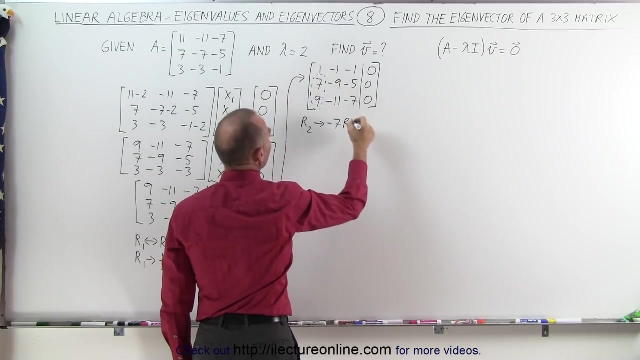 And the top row goes to the bottom: 9, and minus 7, and 0.. Next, we're going to get rid of these two elements by using this one up here. So we take r2 and replace it by the negative of that number, times the row with the 1 in it and adding it to r2.. 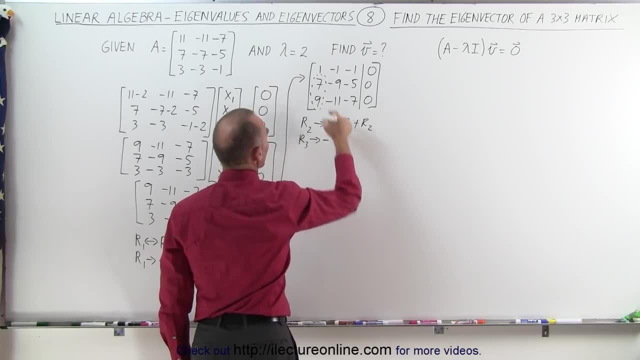 We take r3, the negative of this number, 9, multiply times the row with the 1 in it and adding it to r3.. When we do that, we get the following matrix: The first row doesn't change: 1, negative 1, negative 1, and 0.. How about the second row? 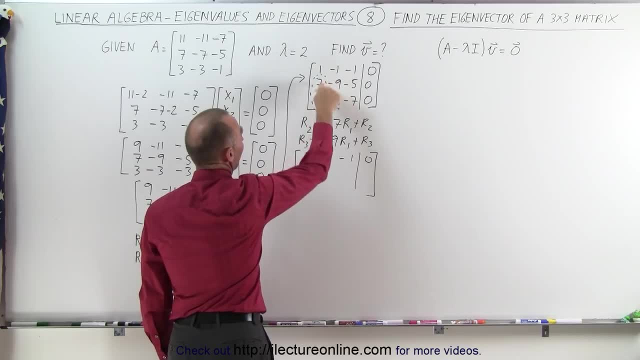 Well, that's the technique. here We have minus 7 times this, added to this, gives me 0.. Minus 7 times this is a plus 7,. added to minus 9 is a minus 2.. Minus 7 added to minus 1 is plus 7,. 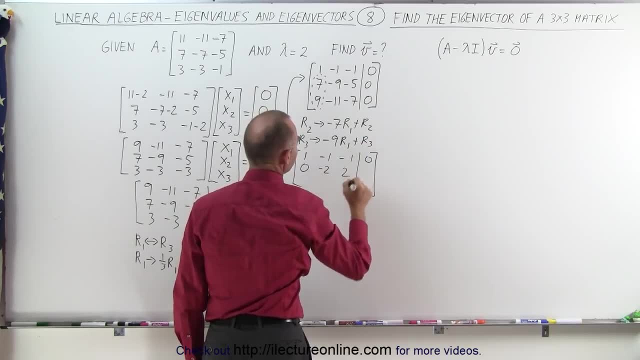 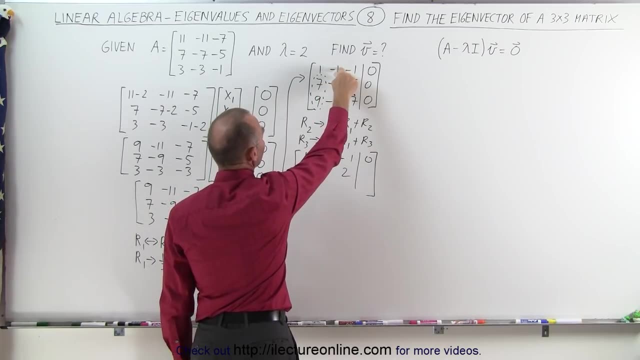 added to minus 5 gives me a plus 2.. For the third row: minus 9 times this. added to this gives me 0,. minus 9, that's a plus 9,. added to minus 11 is a minus 2.. Minus 9 times this is a plus 9,. 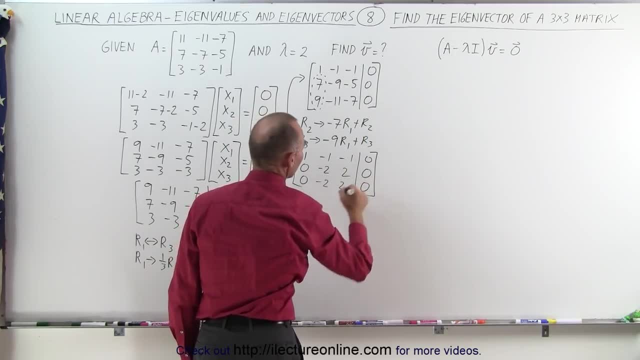 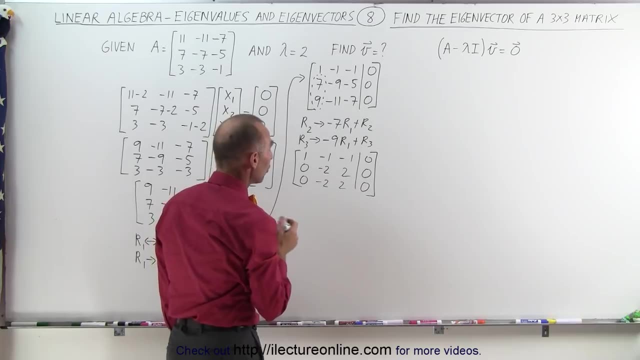 added to minus 7 is a plus 2.. And of course, we have zeros there. Now notice that the two bottom rows are identical. Hmm, okay, So what I can do here is I can make it simpler and divide both of these rows by 2.. So I'm going to take row 2 and make it one half row 2.. I'm going to make 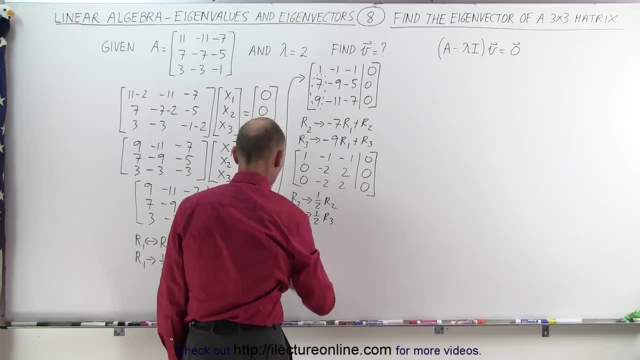 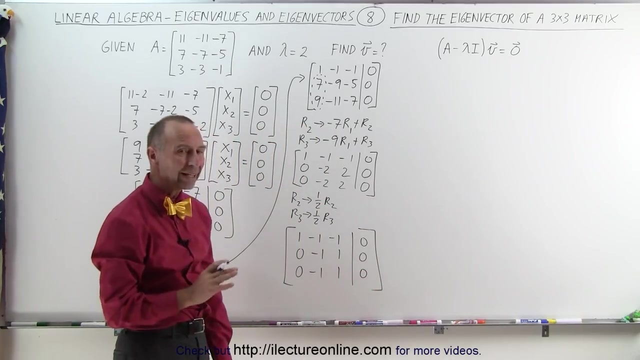 and make it 1, half rule 3, so the matrix looks a little bit simpler like this. so we end up at a: 1 a negative, 1, a negative, 1, 0, 0, negative 1, 1 and 0 and 0 negative, 1, 1 and 0. so writing that now: 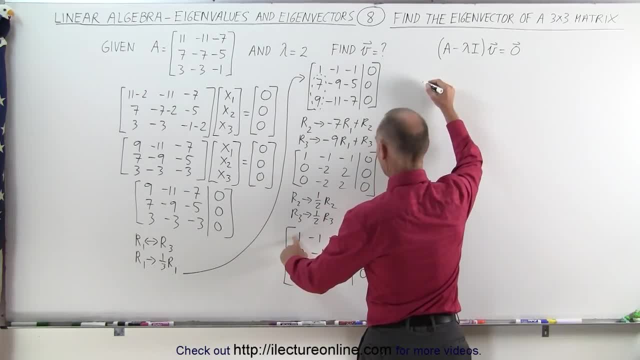 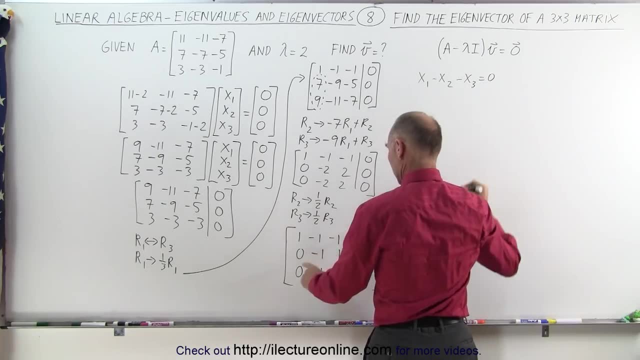 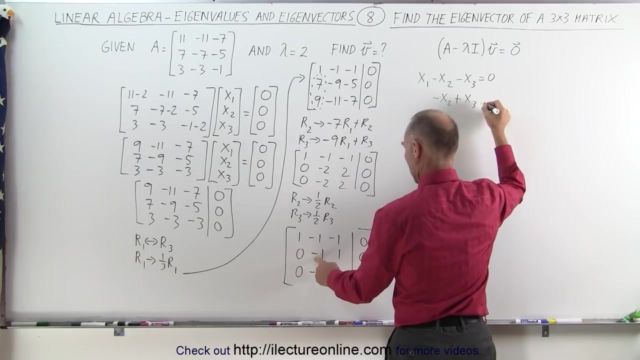 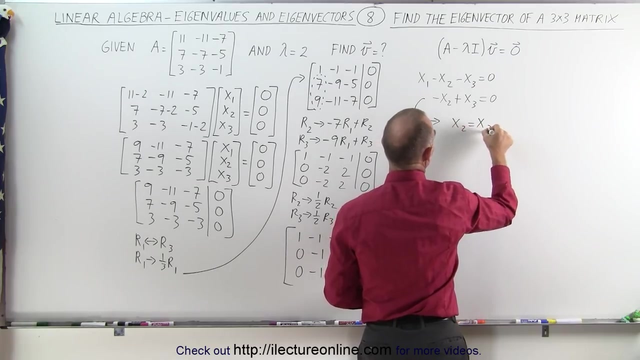 in equation format. using the top, I can say that x1 minus x2, minus x3, equals 0, and from the second equation, which is identical to the third equation, I can write: minus x2 plus x3 is equal to 0. and from the bottom equation, I can simply say that x2 equals x3. so I'm going to do is I'm going to let. 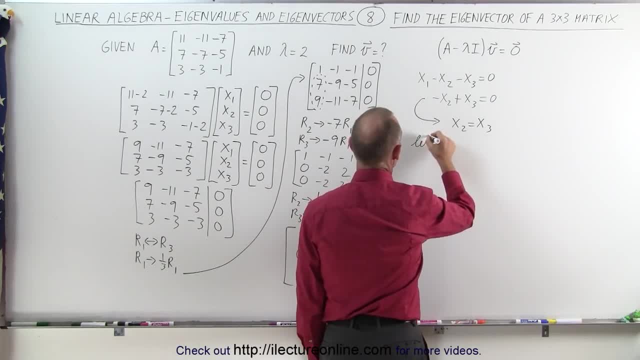 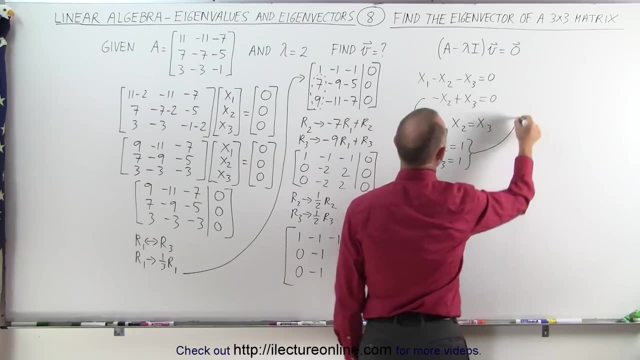 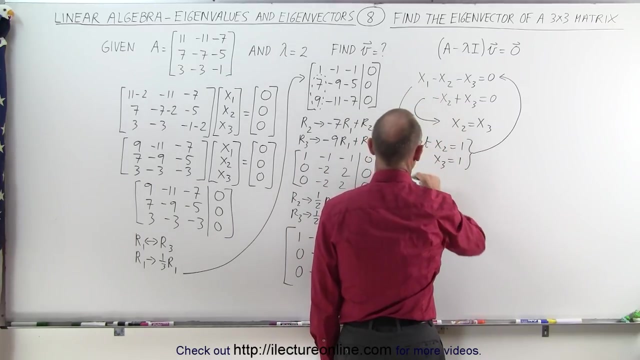 x2 and x3 equal 1. so I'm going to let x2 equal 1, let x3 equal 1, and when I do that I plug those two values back in the first equation to then find a corresponding value for x1. Here I can say that when I take this equation I can say x1 minus x2. 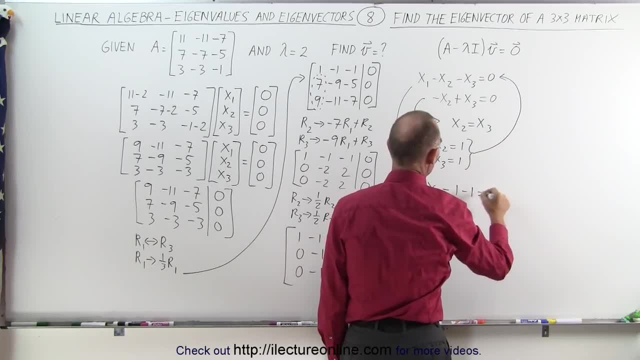 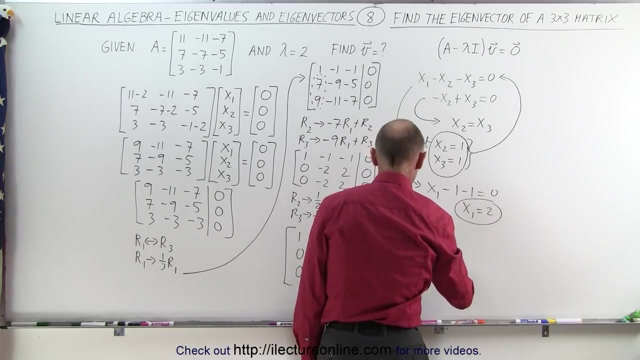 which is 1 minus x3, which is 1, adds up to 0, or x1 equals 2.. In other words, when I let x1 and x3 equal x2 and x3 equal 1, then x1 becomes equal to 2, which means my vector that I'm looking for. 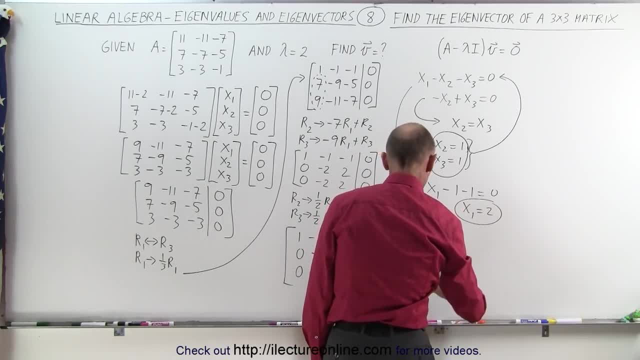 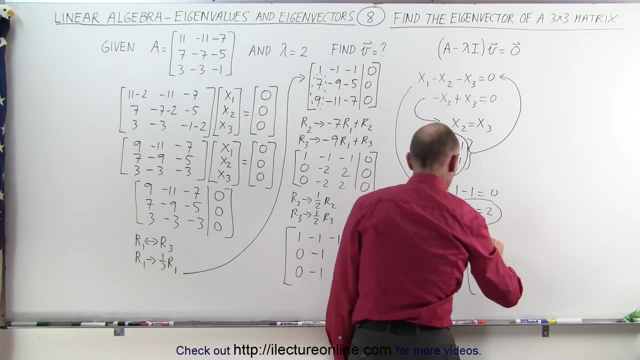 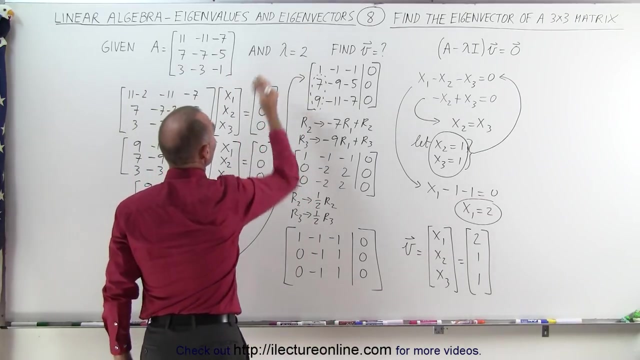 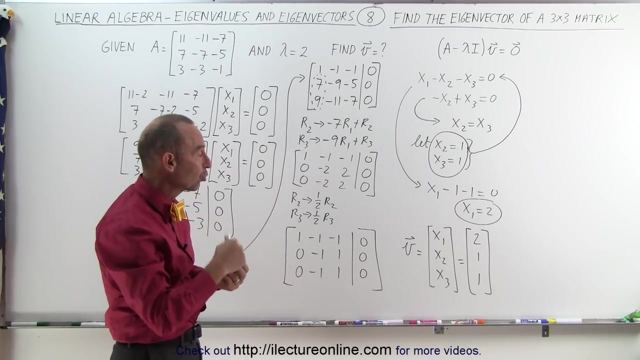 is equal to well, that would be the three variables x1, x2, x3, which then can be written as 2, 1 and 1, and that is the appropriate eigenvector for this matrix. with this eigenvalue, Sometimes we want to normalize the vector, with other words, we want the sum of the squares. 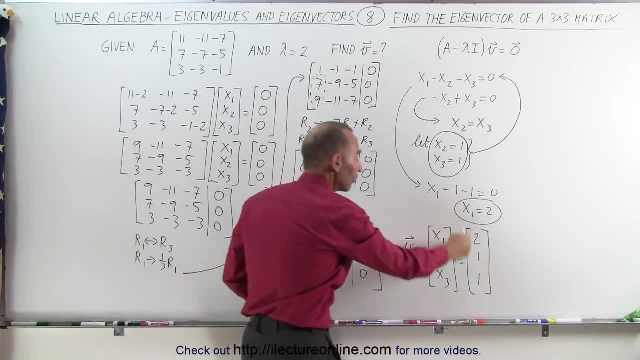 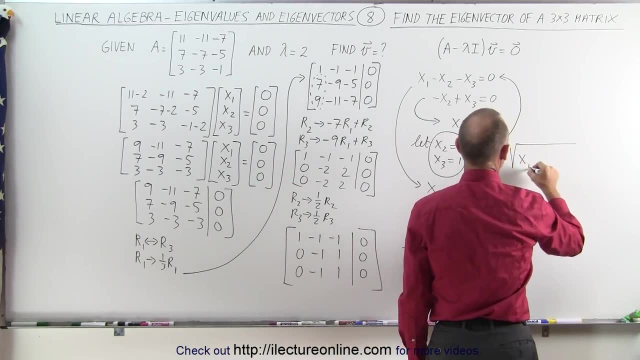 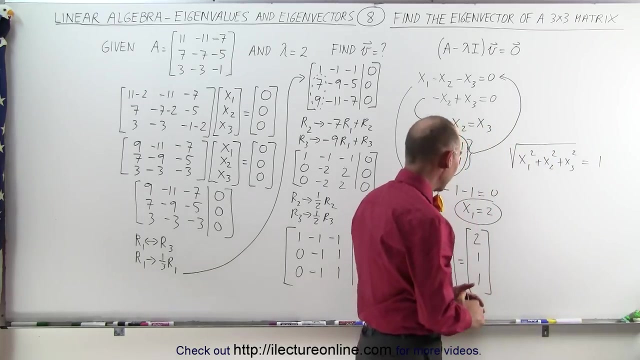 the square root of the sum of the squares of the components of the vector to equal 1.. In other words, what I want is I want the square root of x1 squared plus x2 squared plus x3 squared to be equal to 1.. So I don't know at this point what the values are for x1, x2 and x3. 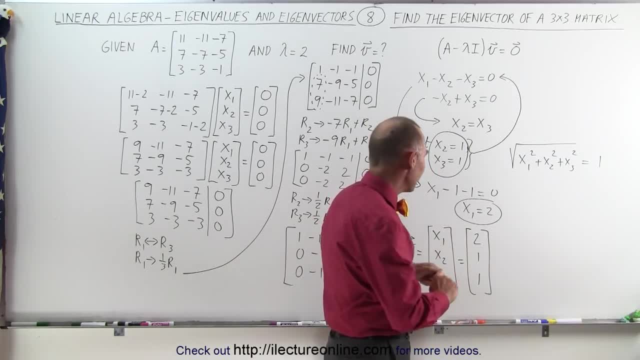 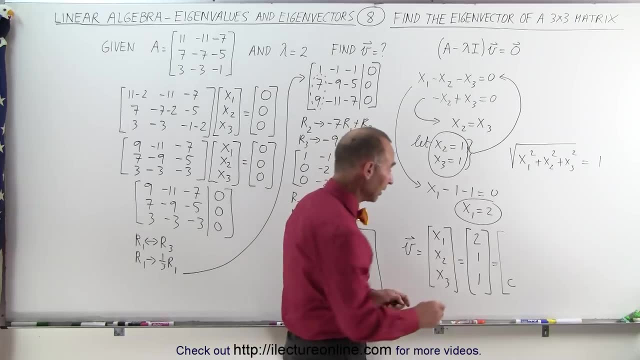